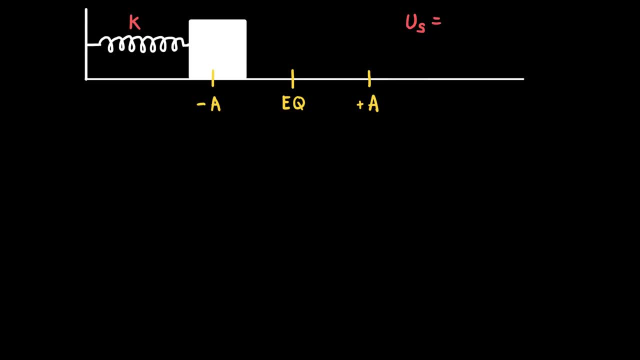 And I know that the equation for the elastic potential energy that's stored in that spring is in general equal to one-half k. That's equal to k- x squared, where x squared represents how far the spring has been stretched or compressed. At the equilibrium position, the spring is at what we will call its rest length. 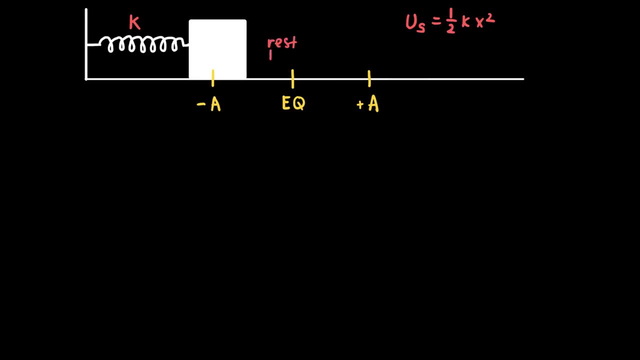 So the rest length occurs at the equilibrium position. It's important that you know I'm defining the equilibrium position as the place where the center of mass of this block would be at, when the system is at rest. So say I let go, and the system oscillates back and forth and eventually it stops. 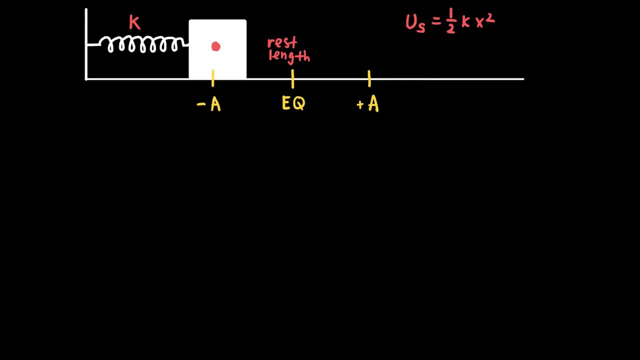 The center of mass of that block would stop at the equilibrium position And when that happens the spring would be at its rest length- It's not compressed or stretched at all- And in that case the x value in my elastic potential energy equation would be zero. 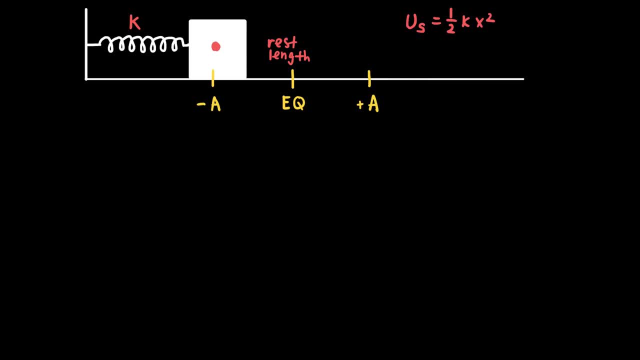 There would be no elastic potential energy in the system, because the spring is not stretched or compressed, But at the position as I've drawn it there in the picture, it is a distance a away from the equilibrium position. So if I wanted to, I could express the elastic potential energy as 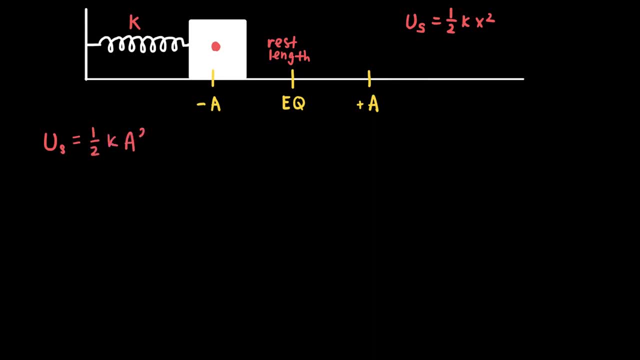 one-half k times a squared, where a is the amplitude that I've given it when I've pulled it back. I also know that the block is not moving and if I define the place where the block is right now to be the place where the gravitational potential energy would be zero, 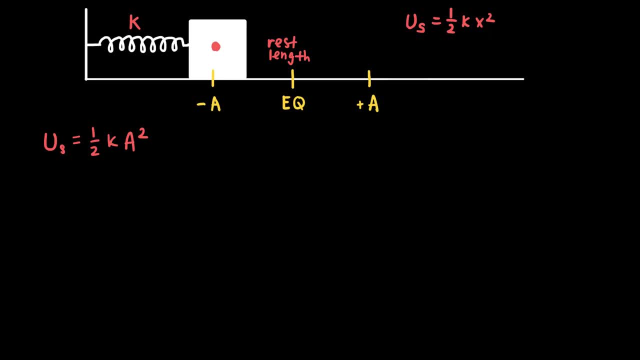 then there's no other energy associated with the initial position of the system as it's drawn there, And so not only is the elastic potential energy equal to one-half k a squared, but that's the only type of energy present in the system, And so for that reason, I'm going to say that the total energy of the system 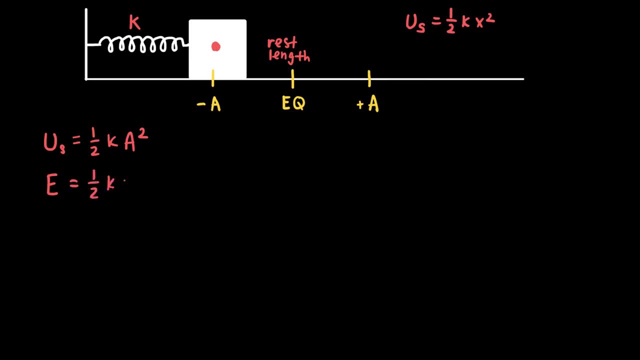 E is equal to one-half k a squared. So in general, for an oscillating system like this, we'll define the total energy of the system E to be related to the initial amplitude that the system has, And so the expression of that equation is one-half k a squared. 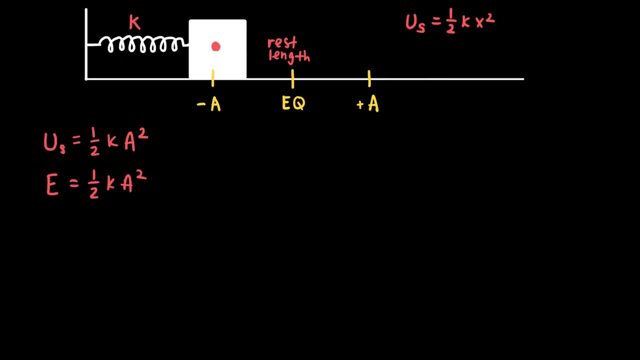 Had I given it an amplitude of two a, twice as much amplitude, then the expression would be one-half k, two a squared, And there would be four times as much energy in the system. So I now know that at the negative amplitude the energy is all elastic potential energy. 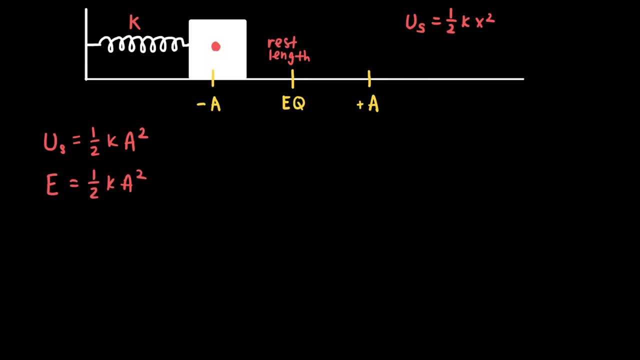 Now let's look at the equilibrium position. At the equilibrium position, the spring would be at its rest length, which means it's not stretched or compressed. That means that the elastic potential energy would be equal to zero. So where did all the energy go? 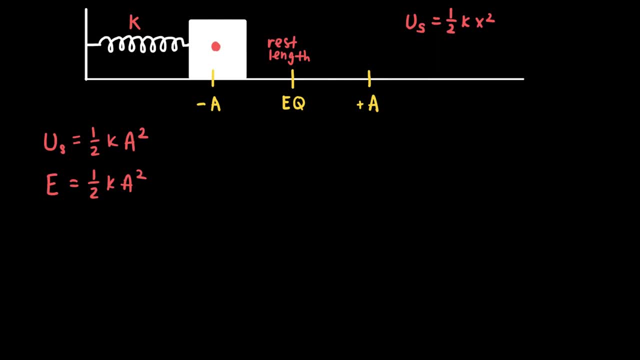 All of that energy now has been converted into kinetic energy. The kinetic energy of the system at the equilibrium position would be equal to one-half m v squared, but not just v squared. I'm going to write v max squared, Because at the equilibrium position 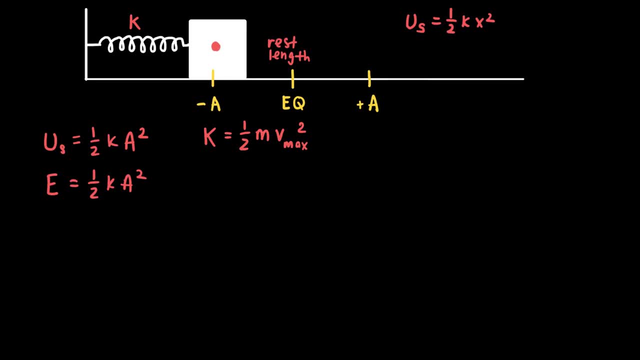 the velocity of this block is its maximum value, And so the total energy of the system could also be written as one-half m v max squared, Because I know that at the equilibrium position the only type of energy present is kinetic energy And, as you might imagine, 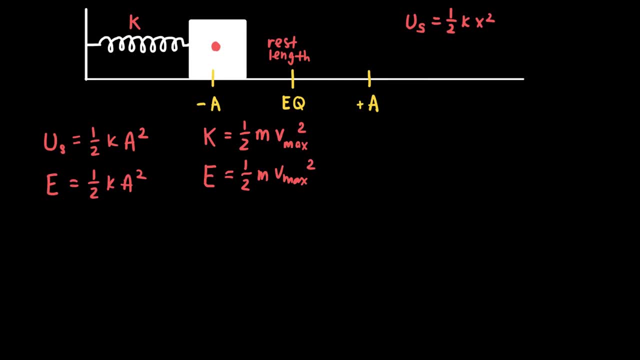 when we move over to the positive amplitude, the same thing is going to be true at the positive amplitude as was true at the negative amplitude. And notice that the distance from equilibrium a here is squared in the equation for elastic potential energy, And so it doesn't matter if we're talking about 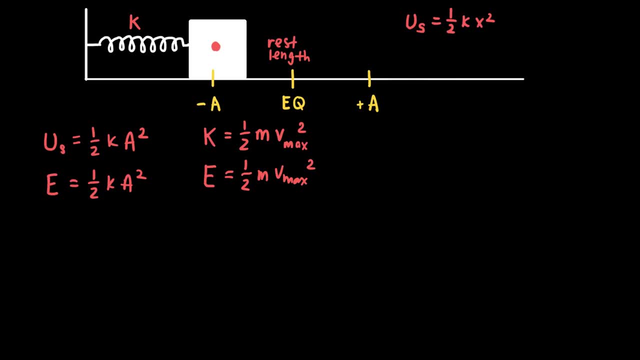 the negative amplitude or the positive amplitude, the energy associated with that position will be positive. And so, at the positive amplitude, I could say that the elastic potential energy is given by one-half k a squared, But I could also say that the total energy 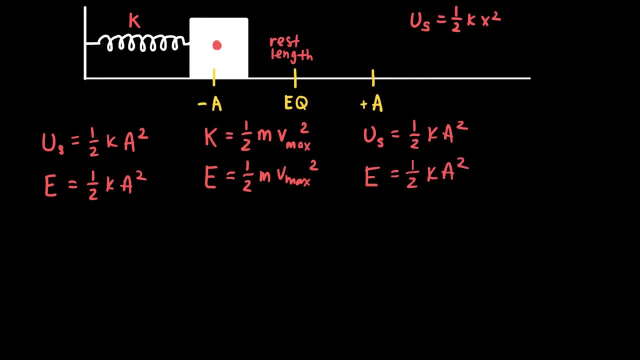 is given by one-half k a squared. So that's what happens at the negative amplitude, the positive amplitude and the equilibrium position. What is true of the energy at a location that is, let's say, one-half a, So minus one-half a. 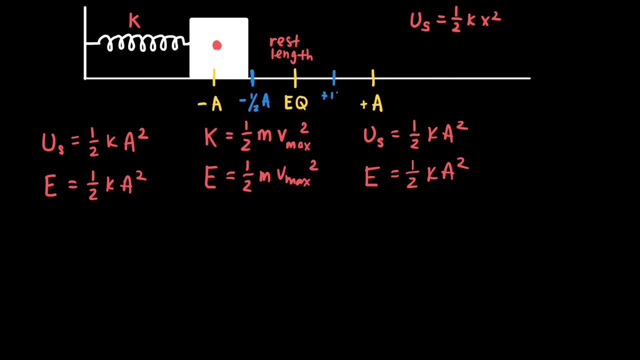 or plus one-half a, You might be tempted to think. well, if it's all kinetic energy at the equilibrium position and all elastic potential energy at the maximum amplitude, then halfway in between we should have half of each type of energy. 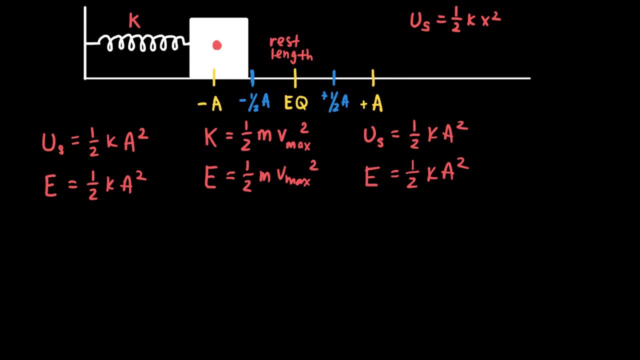 And while that's an incredibly reasonable thing to think, that's completely wrong. And so how can I figure out how much of the energy is kinetic energy and how much of the energy is elastic potential energy at any particular position, like one-half the amplitude? 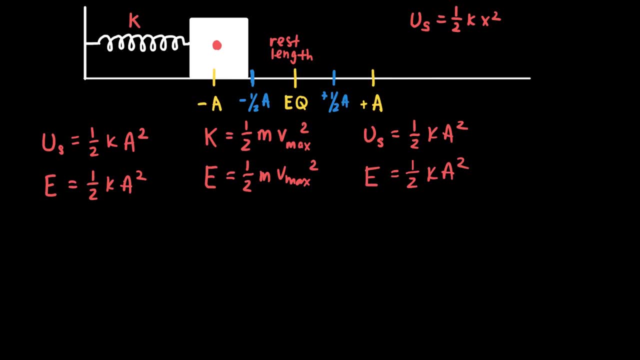 The way that I would show that is the following: I would say that at one-half the amplitude, the elastic potential energy we have in a form of an equation that looks like this: one-half k, but instead of a the amplitude at this location is just one-half a. 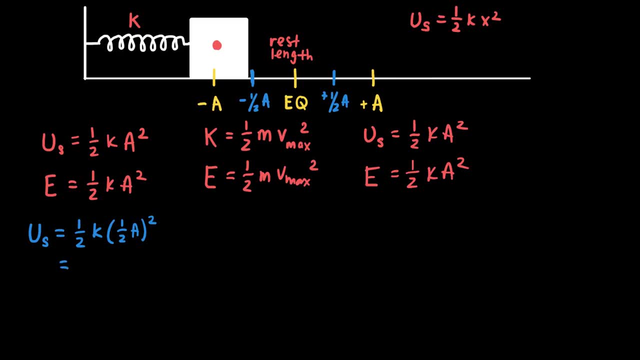 So the elastic potential energy term is equal to- I'm going to write this in kind of a strange way- one-half k, a squared, and then the one-half inside the parentheses would be one-fourth. Okay, I'm writing it in this way. 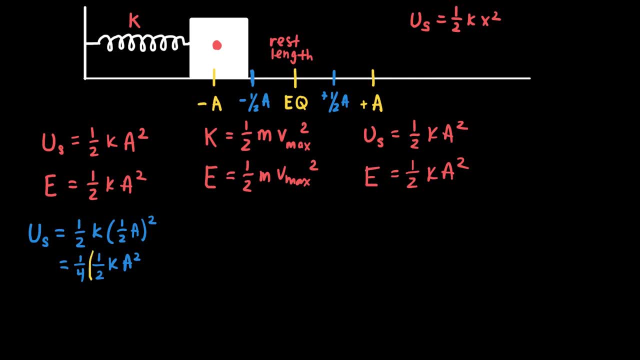 because everything inside the parentheses here, the one-half k a squared, is exactly what I wrote for the total energy at the maximum amplitude, And so if one-half k a squared represents the total energy of the system, then the way I can express the elastic potential energy is: 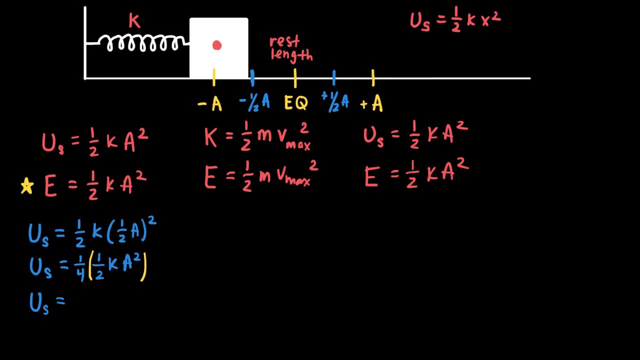 the elastic potential energy at one-half a is equal to one-fourth of the total energy. So the elastic potential energy at one-half the amplitude is equal to one-fourth of the energy. If that's true, then how much of the energy is kinetic energy? 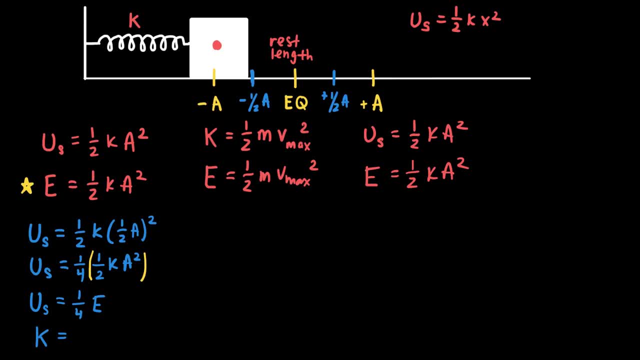 If one-fourth of the total energy is elastic potential energy, then that means that the other three-fourths of the energy must be kinetic energy, And so at either one of those positions, at half the amplitude, 75% of the energy is kinetic energy. 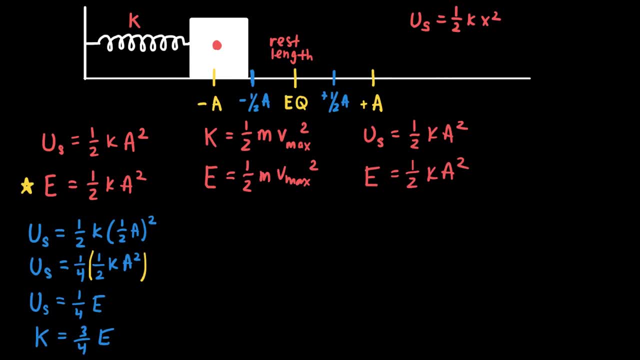 and 25% of the energy is potential energy, And one reason why I know that to be true is because, at any moment in time, so long as no energy is being removed from the system, the total energy needs to remain constant, And so I see here: 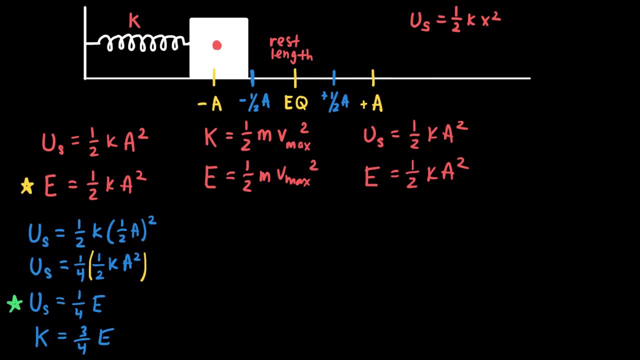 that the two terms that I just wrote, the elastic potential energy is one-fourth of the total energy and the kinetic energy is three-fourths of the total energy. those two terms would add up to the total energy: E, One-fourth E plus three-fourths E. 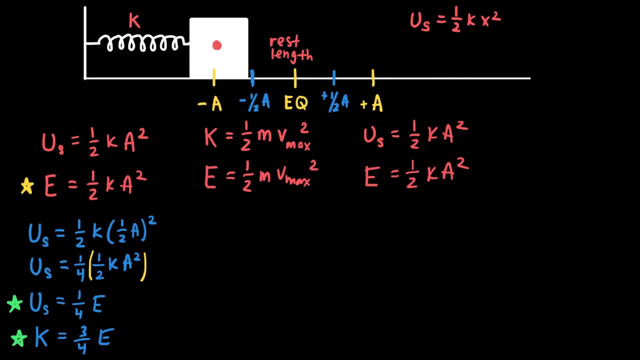 is just E, which is equal to the total initial energy that this system had when I pulled it back to its negative amplitude. So now I'd like to go ahead and look at a graph of the energy as a function of position for this system. 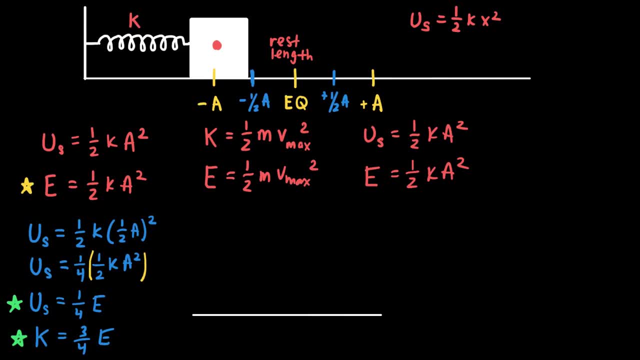 What would that look like? And so we're going to make a little graph with just one axis that has, at each point, the energy that's associated with that position. So I know, for example, that at the negative amplitude all of the energy is elastic: potential energy. 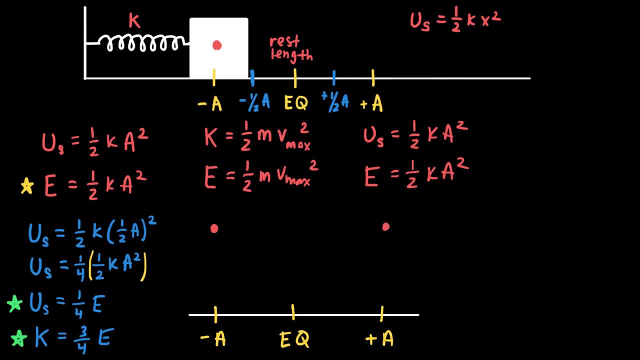 At the positive amplitude, all of the energy is elastic potential energy, And at equilibrium, the energy in the spring is zero, And so this red line I'm going to draw is associated with the elastic potential energy, And I know because the elastic potential energy 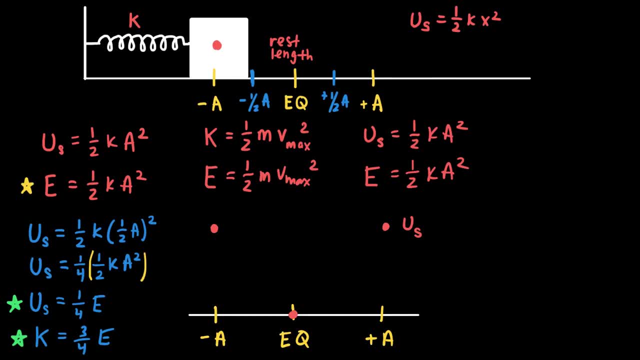 is proportional to x squared, the position, or that stretch, distance squared, then the relationship between these two things will be parabolic. And so my graph looks something like this: where on either side of the equilibrium the elastic potential energy increases in that parabolic kind of fashion. 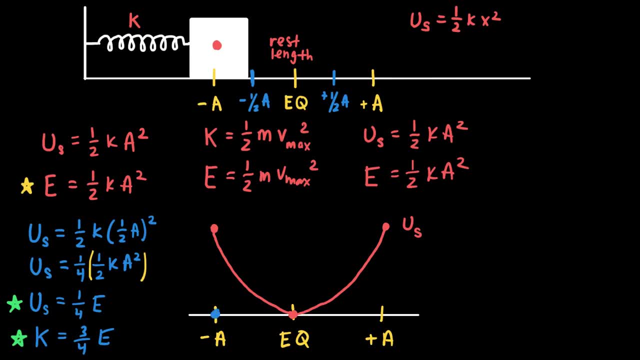 Now for the kinetic energy. the kinetic energy at either amplitude will be zero, because as it approaches either amplitude it slows down before stopping and then turning around and going in the other direction. But then, at equilibrium, the kinetic energy will be a maximum. 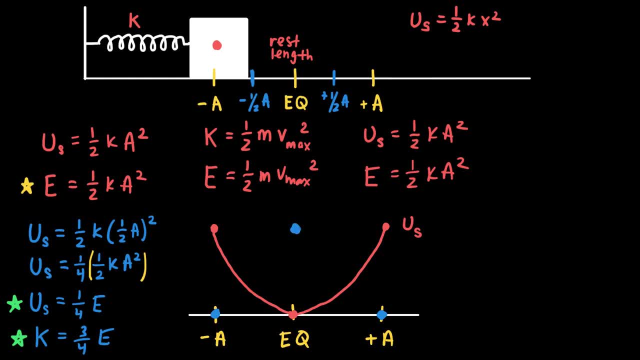 but not just some arbitrary maximum value. It will be an amount of kinetic energy that is equal to the amount of elastic potential energy that the system had when it was at its maximum amplitude, And so this graph is also parabolic, as it increases, as it gets toward equilibrium. 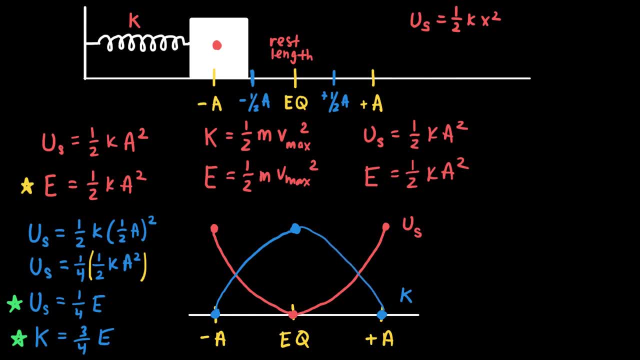 and then decreases as it moves away from equilibrium. And so what we find is that if we choose, for example, that position of one-half A, then- although my graph is poorly shown- if we were more careful about this, we would get closer to the relationship. 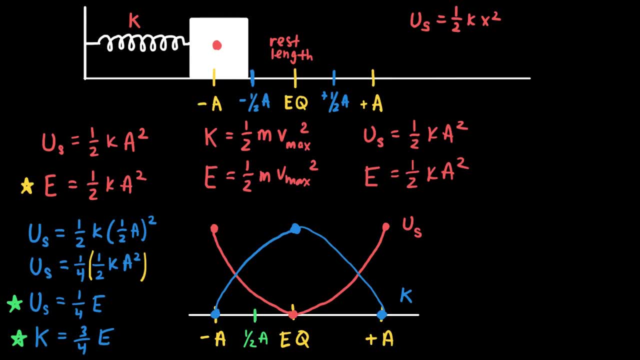 that I've shown on the left there, but the potential energy is quite low And the kinetic energy is much higher than that. Now, perhaps this graph isn't the best evidence of proving that 25% of the energy is elastic potential energy and 75% of it is kinetic energy. 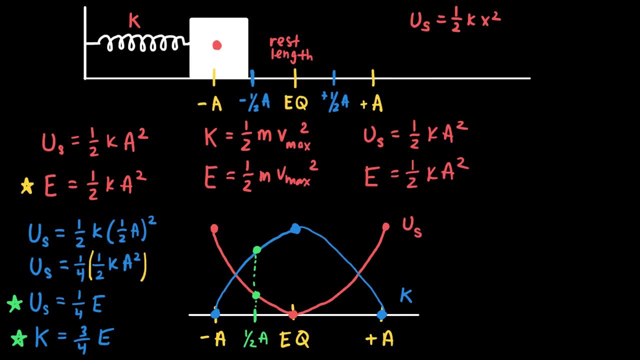 but that's something you could measure for yourself. But given the relationships that I have here, at least you can see, even with my poorly drawn graph, that substantially more of the energy is associated with the kinetic energy at half the amplitude. If I wanted to draw a line. 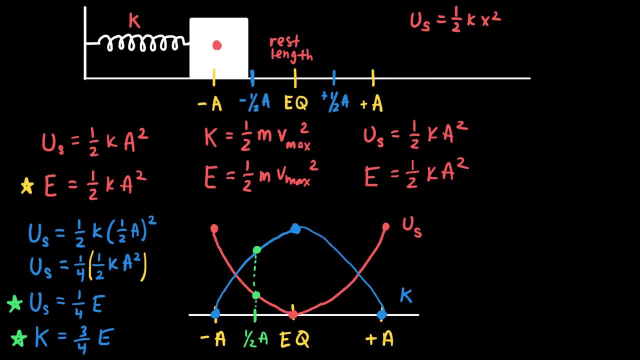 that represented the total energy as a function of time, then it would probably look something like this: right, It would start here and it would just be a horizontal line that continues on, And so perhaps that line represents the total energy which would stay constant. 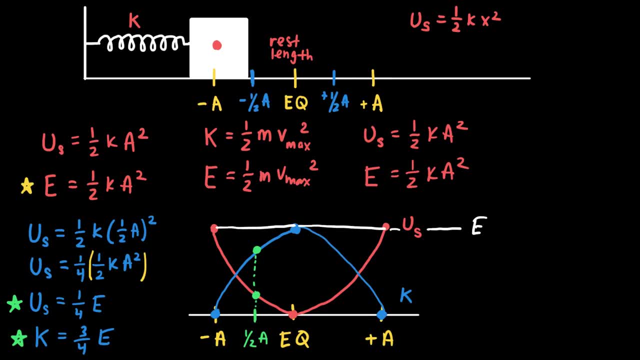 And so how could I summarize all of what we're learning here in a useful kind of way? The energy at any particular moment in time- so not particularly the points that I've addressed here, but just any arbitrary point- would be equal to 1 half kx squared. 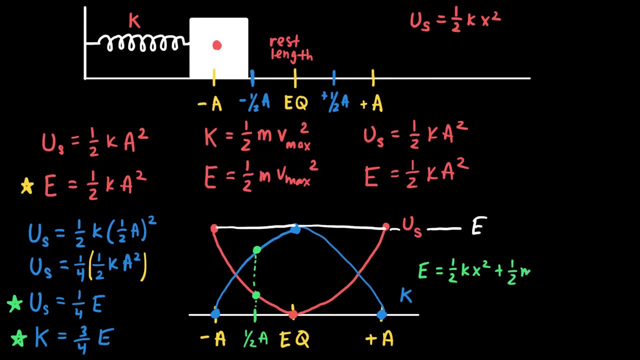 the potential energy at that location plus 1 half mv squared. whatever the kinetic energy is at that location And in terms of problem solving, if I look back to the initial equation that would describe the total energy of the system, notice how, so long as that block, 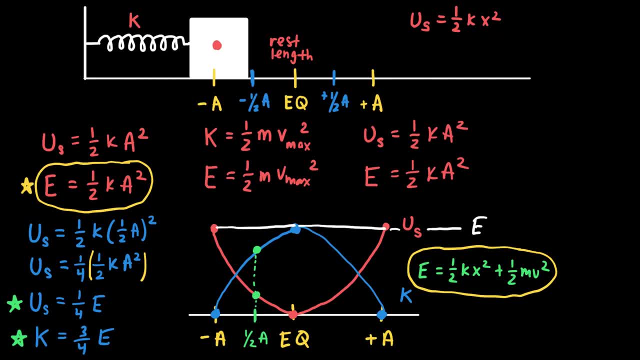 is on a frictionless surface, none of that energy is being removed, So at all moments in time, if I just know that initial amplitude and the spring constant, then I could very quickly calculate a number using that equation: 1 half k a squared. 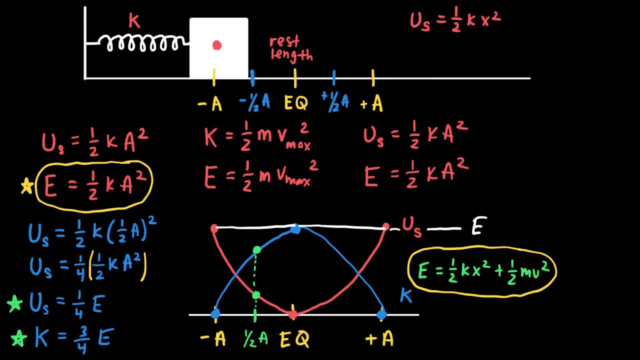 And that number would represent, in joules, the amount of total energy present in the system. And so if I knew that number, you could imagine using the equation that I've written here and setting that number which represents the total energy. 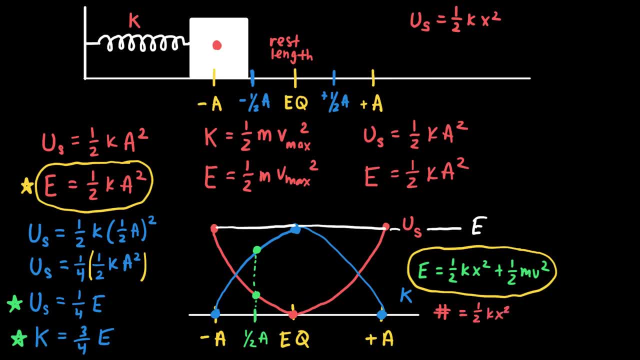 equal to 1 half kx squared plus 1 half mv squared And, for example, in a problem being given some arbitrary position, right so when the system is 1 centimeter away from equilibrium, or when the system is 1. seventh, 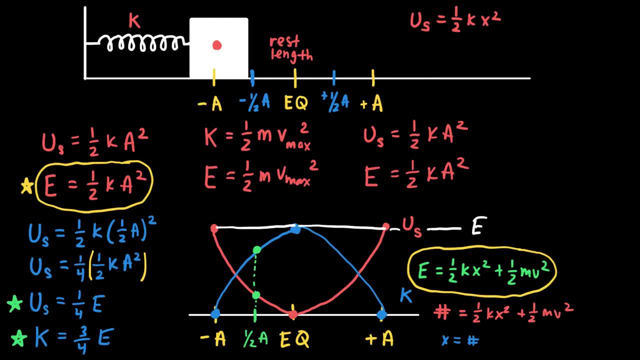 of its amplitude away from the equilibrium, and using that number, and using the number for the total energy to solve for, for example, the velocity, And so I could determine how fast the system would be moving at a particular location, knowing things like the mass of the block. 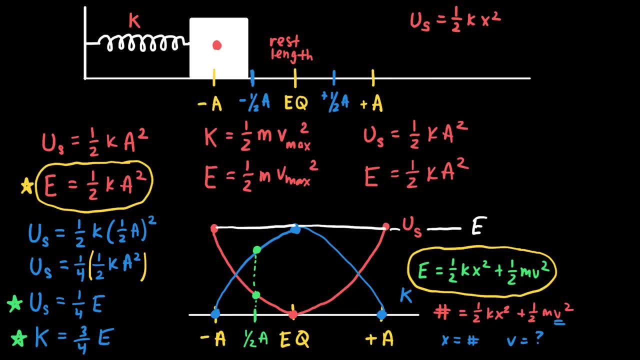 the spring constant and using the initial amplitude to determine the initial total energy. I would also like to reiterate the idea that this calculation that I've shown on the left in blue is an extremely important kind of calculation. I can always express either type of energy. 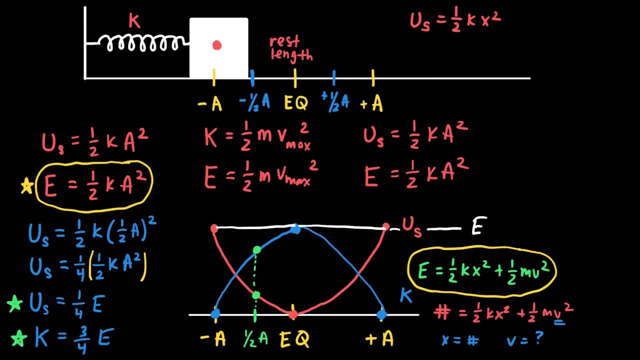 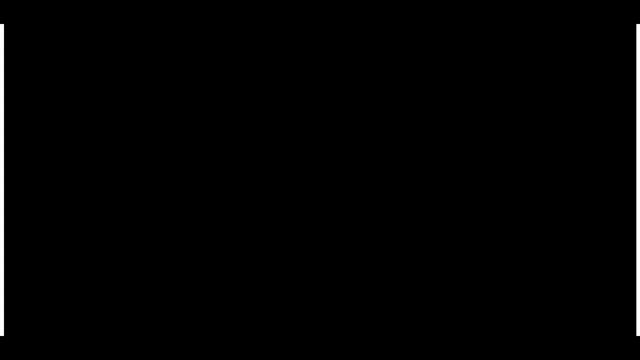 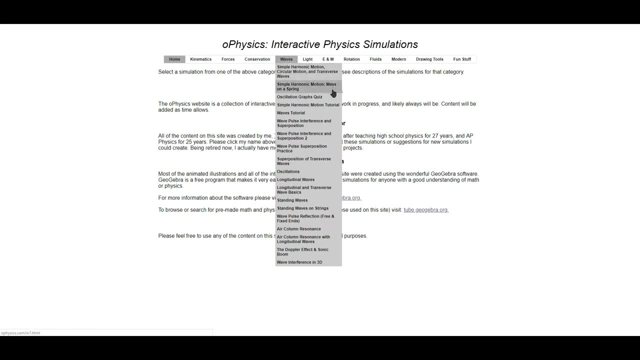 as a fraction of the total energy, which can be expressed as 1 half k a squared. It's crucial that we understand that. Lastly, I'd like for you to go to oPhysics, spelled as it is at the top of the website title there.